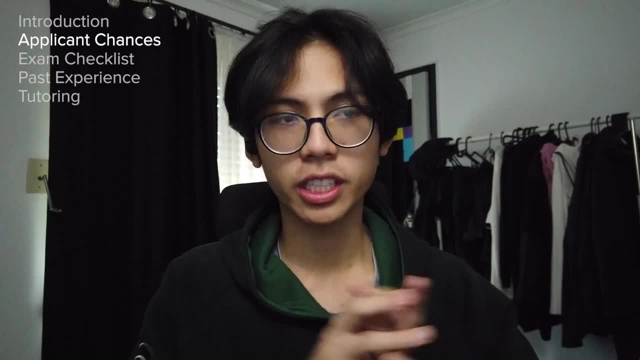 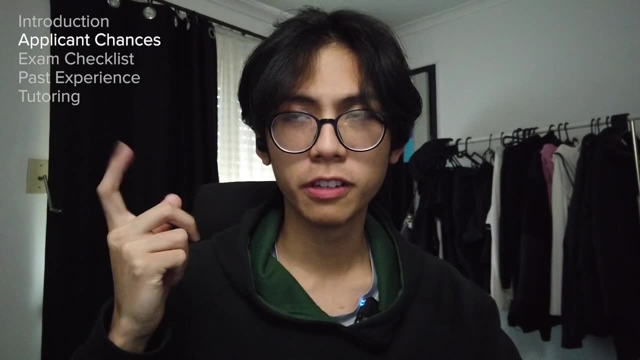 under the assumption that it's an even split of 1,500 male applicants and 1,500 female applicants. The application process for year 8-9 is just the exam, but if you're applying for a year level above, there's also an additional interview stage that you must do: The examination for the selective. 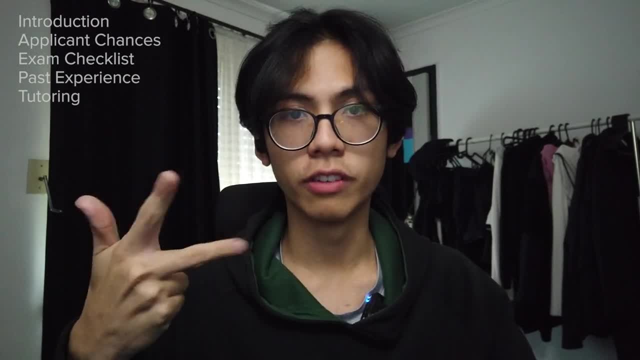 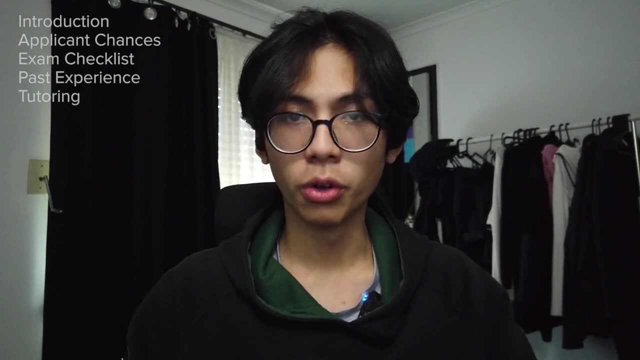 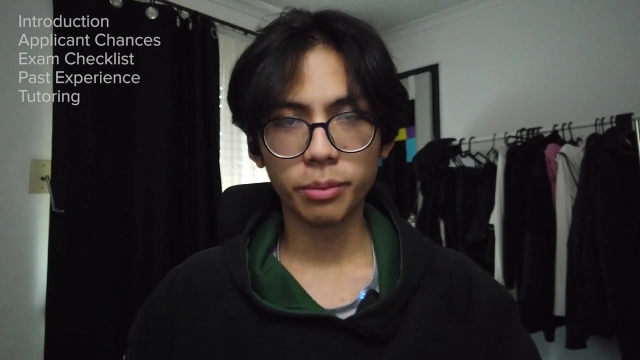 schools is under five topics: mathematics, reading comprehension, verbal reasoning, numerical reasoning and a creative or persuasive writing. The four non-writing exams are undertaken in 30 minutes and are all multiple choice. Further details will be discussed later. I've created a mini checklist outlining all the skills and 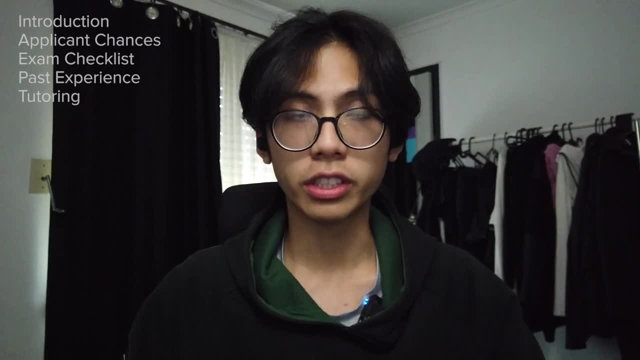 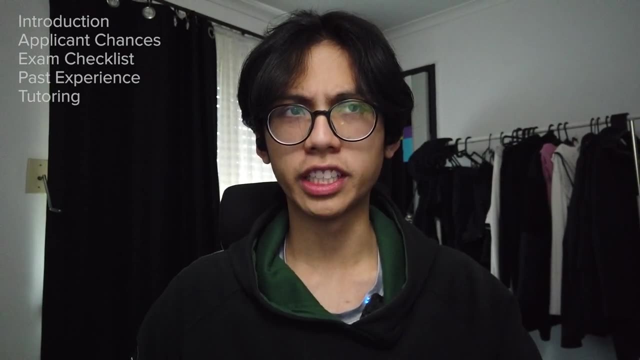 question types that will appear on the examination, so feel free to open that up and follow along as we go over that. now, As we're going through the checklist, I will include a couple questions that I've created in my practice exams. Mathematics comes under around 16 topics, but 14 are mainly. 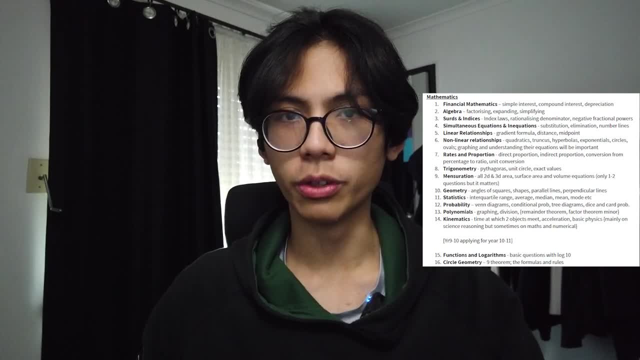 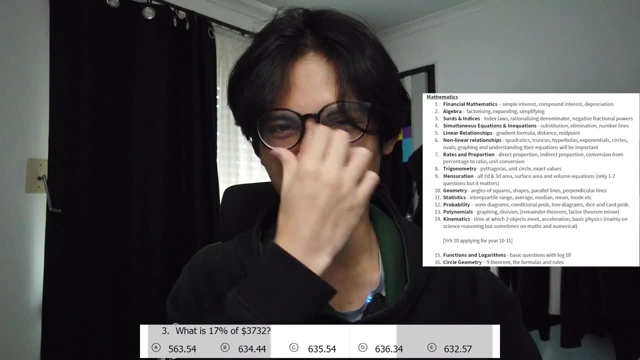 for the Main Year 8-9 exam. The last two are more relevant for those in higher or older year levels. Number one: financial mathematics. So know simple interest, compound interest and depreciation. Number two: algebra. Know how to factorize, expand and simplify. 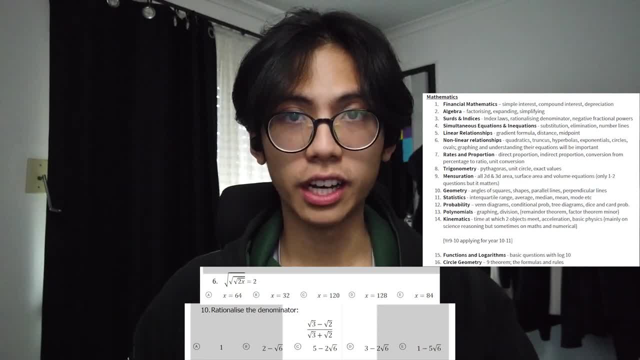 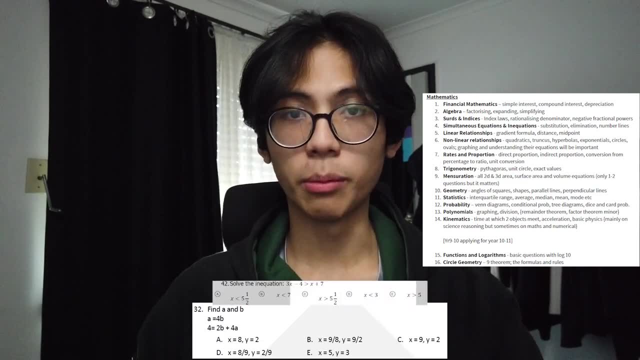 Number three, thirds and indices. Know your index laws, how to rationalize how negative powers work as well as how thirds work, because that's a very important part of your exam. Next is simultaneous equations and inequations, so know how to use the substitution method. 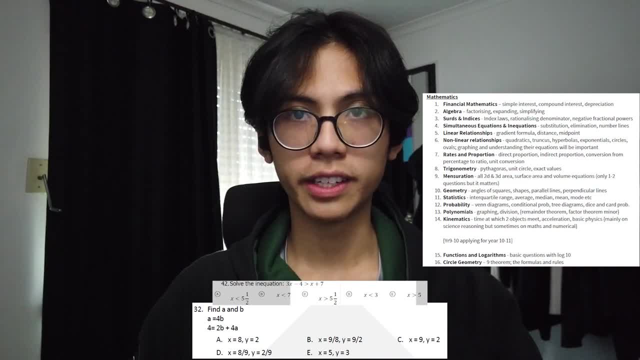 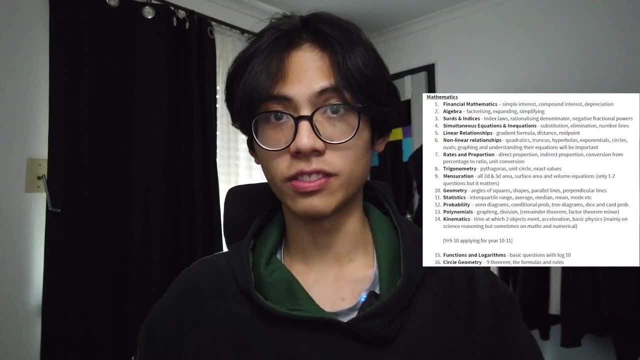 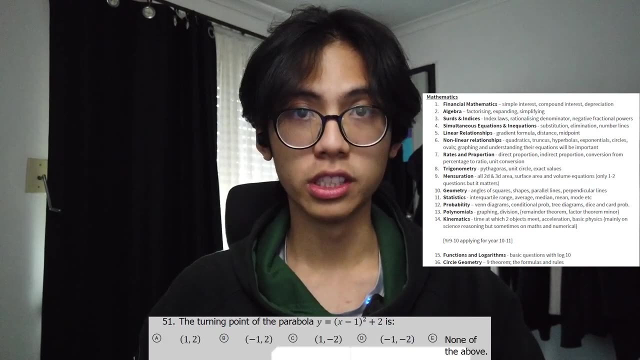 elimination method, as well as how numbers work on the number line. then we have linear relationship, so the form y equals mx plus c. gradient formula, midpoint formula, distance formula- just know all of those and you'll be good. then we have non-linear relationship, which includes quadratic hyperbolas. 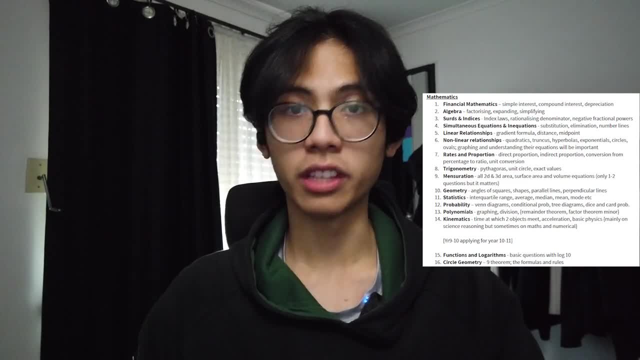 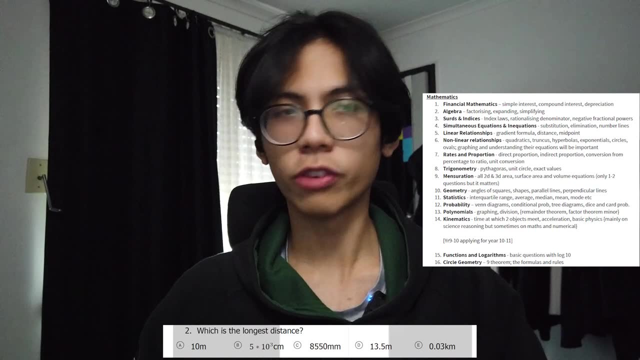 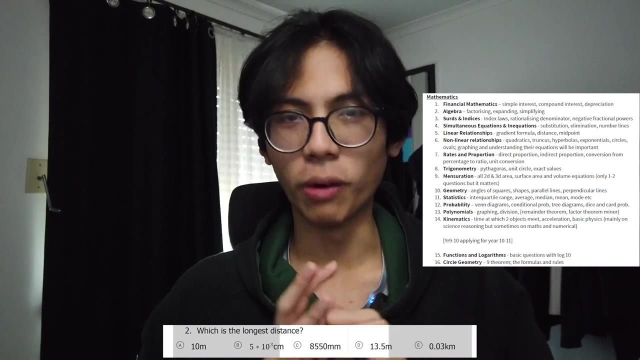 exponential circles, ovals, and how to graph them and understand their equation. next we have rates and proportions, which talks about direct proportion and indirect proportion, as well as like conversion from percentage to ratio, as well as just general unit conversion from millimeters to kilometers. just a whole bunch of those. next is trigonometry, so no pythagoras, unit circle and. 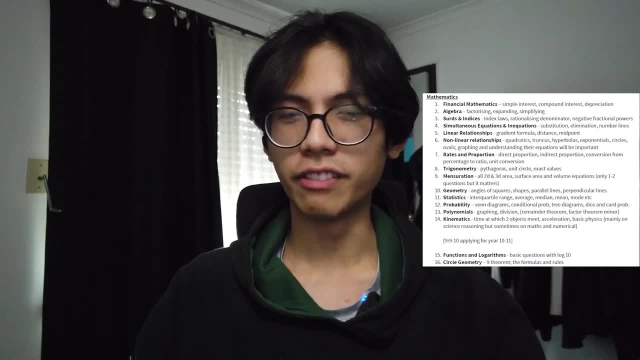 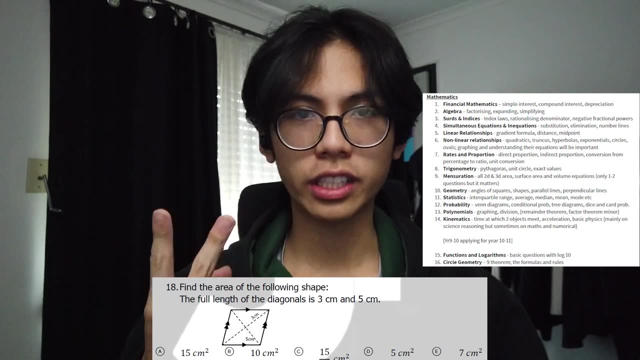 exact values. this is probably around five questions on the exam. then you have like mensuration, which is all the 2d and 3d area, surface area and volume equation. it's only two questions on the exam, one for volume and one for surface area, but it is important that you learn all of them in one of 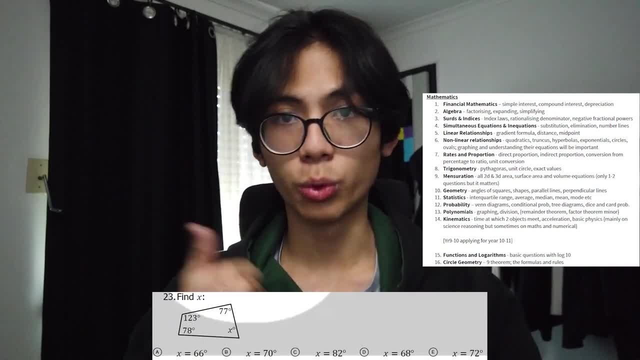 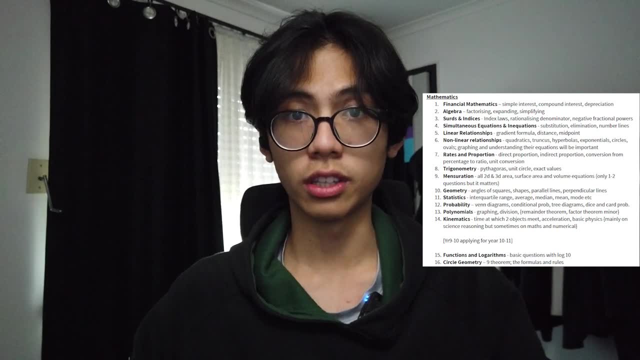 them comes up. next we have geometry, which is geometry, which is the area of the surface area, which is the area of the surface area, which is angles of squares, triangles, circles, parallel lines, perpendicular line, and you're just knowing how to find angles within certain scenarios. next is statistics, or interquartile range, average mode. 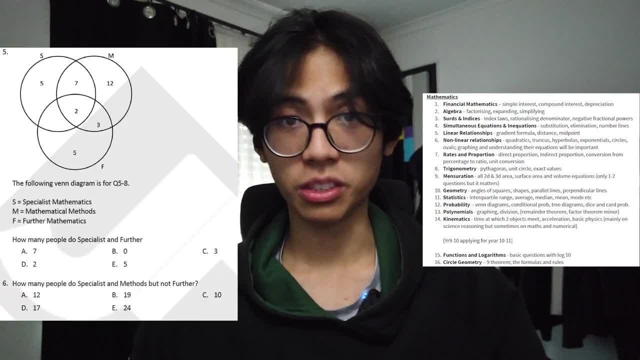 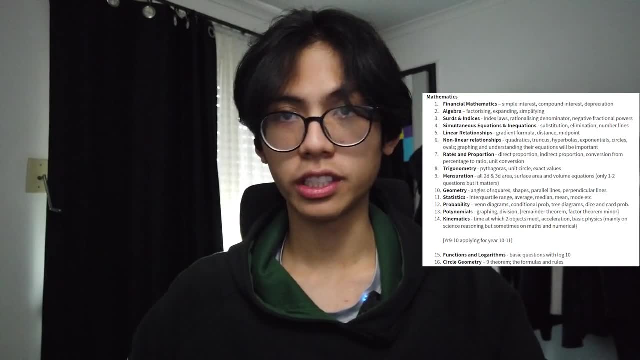 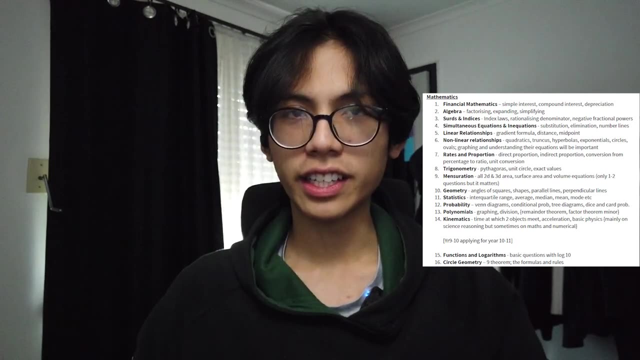 median mean. you need to know all of that. probability is also going to be on the exam. so venn diagrams, conditional probability tree diagrams, how card and dice probability also work, will be handy. next we have two minor soda chapters such as polynomials and kinematics: understanding 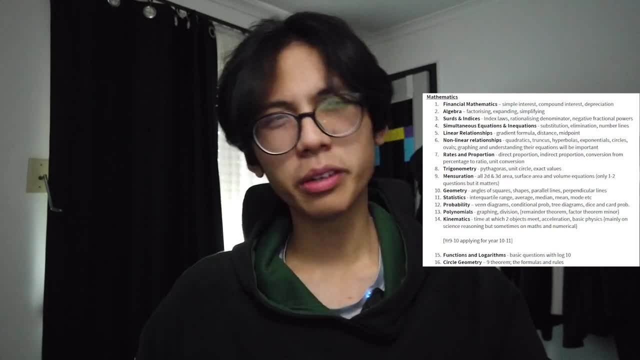 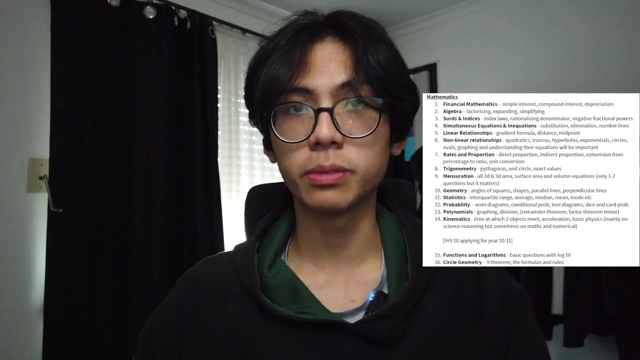 graphing and division of polynomials will be important. factor theorem and remainder theorem aren't really on the exam but might be helpful for those applying for the levels above. kinematics is also one that is more prevalent on the science reasoning exams and the numerical reasoning exams, but it doesn't hurt to know a bit about it in case it pops up. so the main question is the. 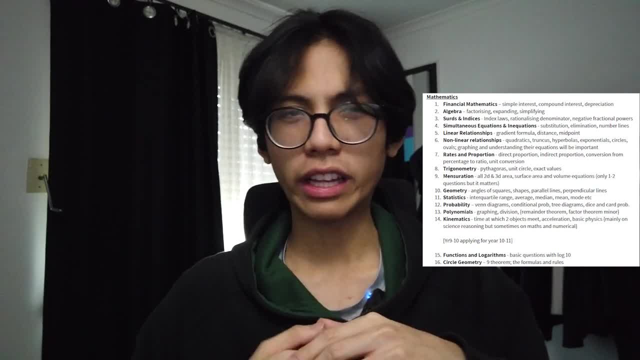 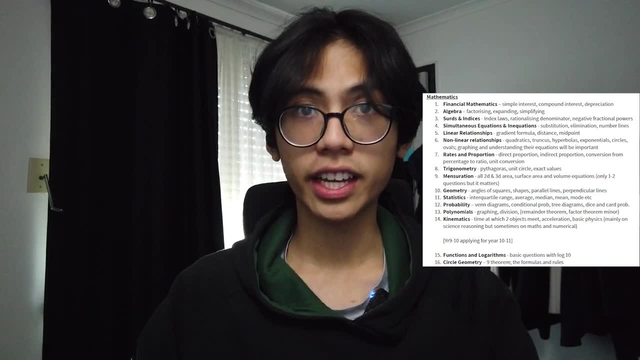 time at which two objects meet will be like a mathematics question, and then knowing like acceleration and a bit of basic physics will also help. okay, so this mainly applies for those applying for years nine to ten, and the math that you're learning will be a bit more relevant if you're 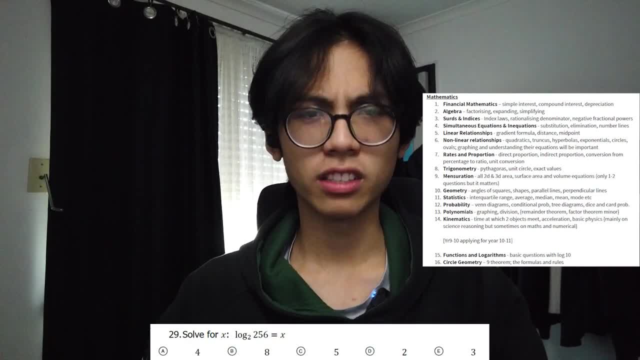 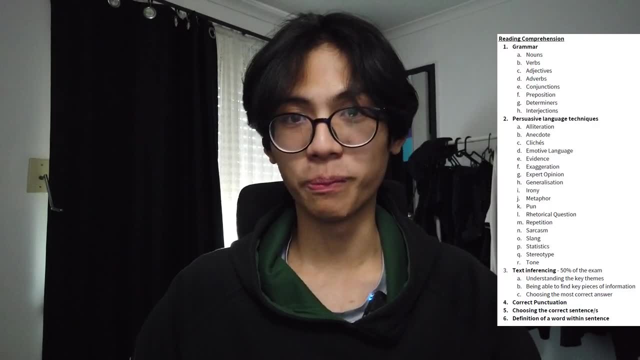 10 to 11. know basic questions with log 10 and circle geometry. know the nine theorems as well as the formula and rules. yep, that pretty much concludes mathematics time for reading comp. okay, i've broken reading comp into six sections. the first two are like the skills that you need. 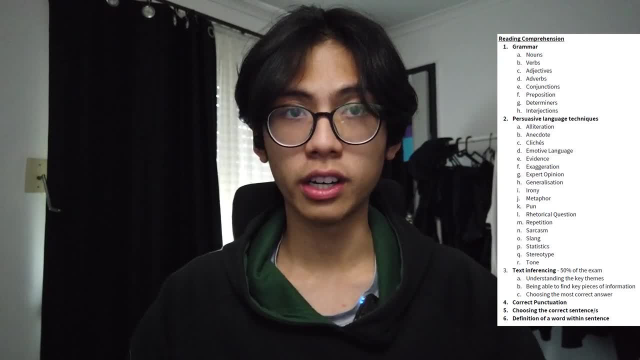 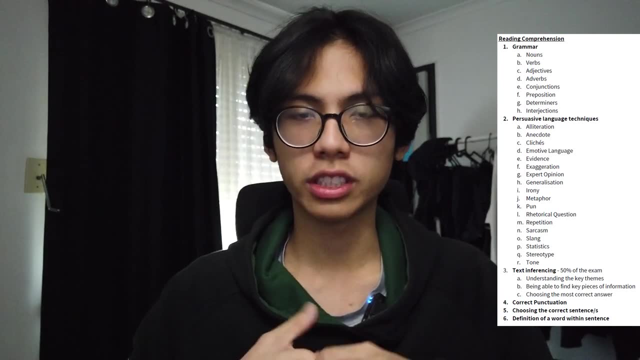 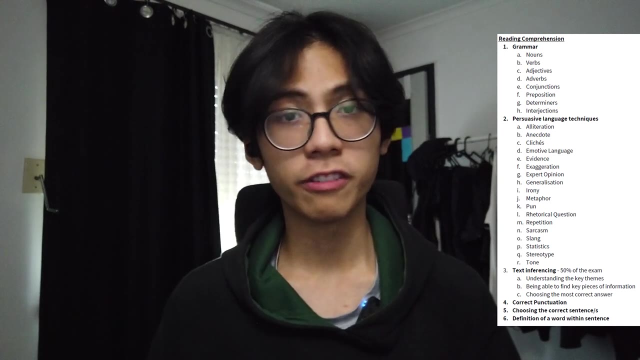 to know before you do your exam. so make sure you know, like all, the grammar as well as persuasive language techniques, because they tend to ask a lot of grammar related questions, as well as which persuasive language techniques are used within certain tech. the next component is text inferencing, which is around 50 of your exam. so, out of the 50 or so questions you're going to be asked, 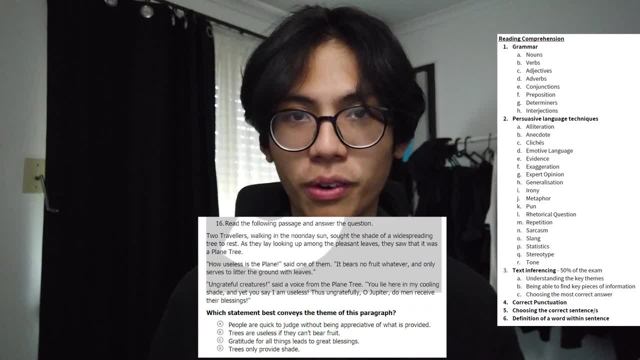 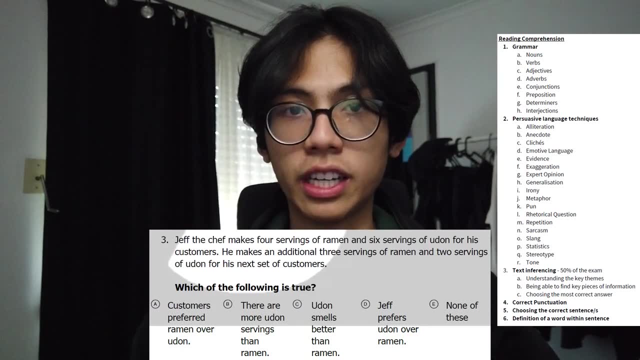 answer the questions around the text, and they're all meant to be performed under 30 seconds, so knowing how to read faster or only find key bits of information will help with part of the exam. knowing correct punctuation is next, as well as choosing the correct sentences for certain. 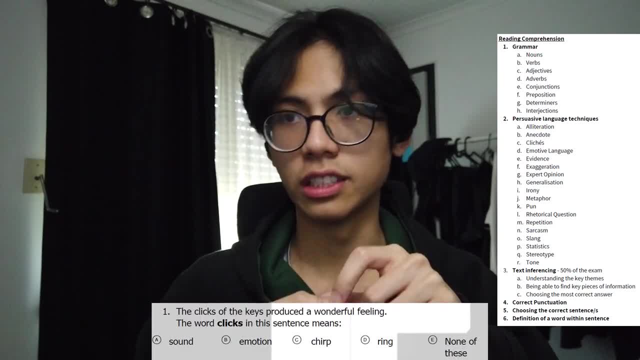 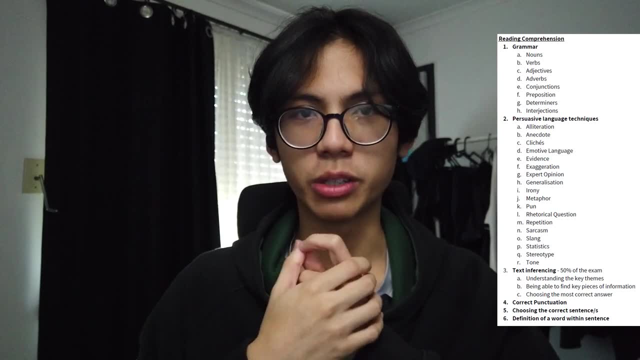 scenarios and knowing the definitions of words within a sentence. this will help you to know the correct punctuation and the correct sentences, for certain scenarios will be mainly inferred by words that are around the like set word. and yeah, that's pretty much the whole of the reading comp exam. so we have verbal reasoning. verbal reasoning is broken up into three. 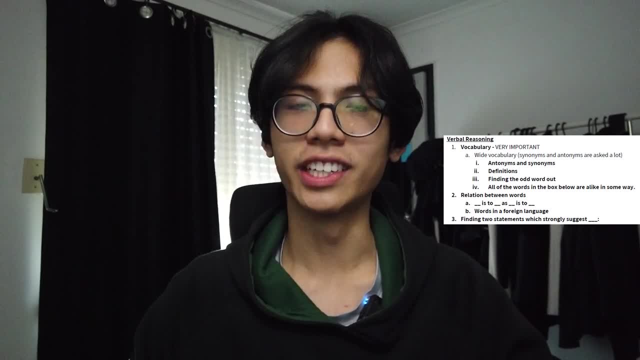 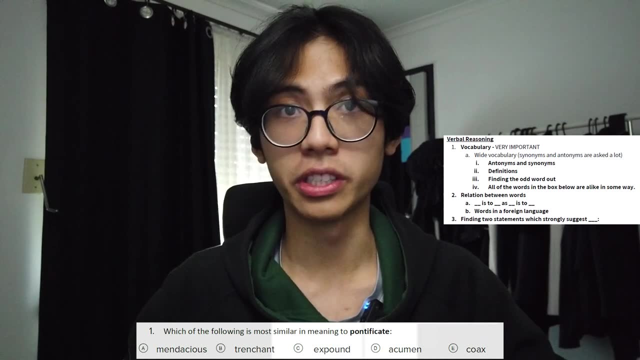 parts, we have the main focus of the exam, which is vocabulary. if you don't have a wide vocab, you're actually going to spend majority of the time guessing, and that's not really helpful. if you're, if you're aiming for a superior. so in vocab they're going to ask around antonyms, synonyms. 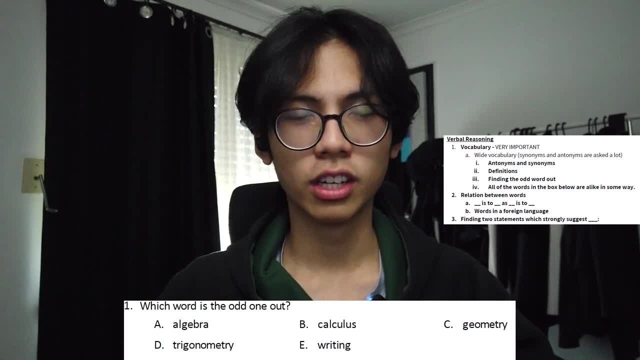 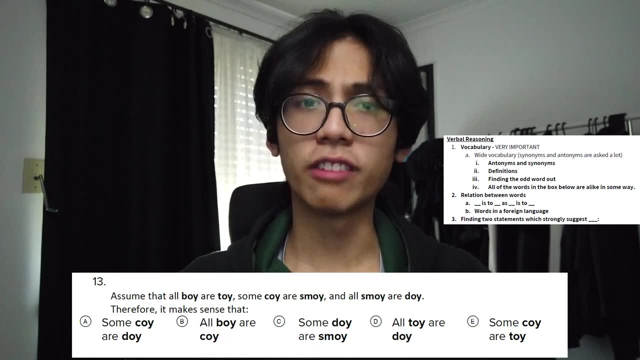 definitions for the word, as well as finding the odd word out and determining like. which word is the odd one out from a box or from the given answers? it really depends. then we have relationship between words. so blank is to blank as blank is to blank. uh, this example here will pretty much 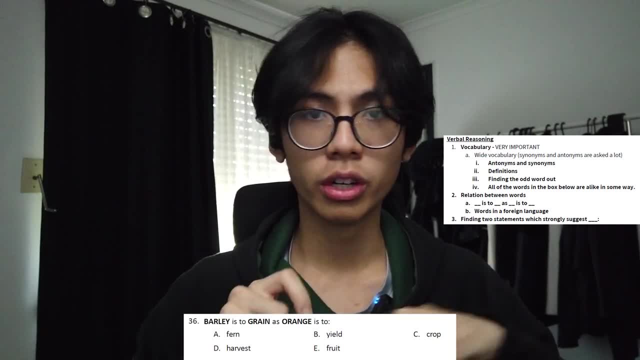 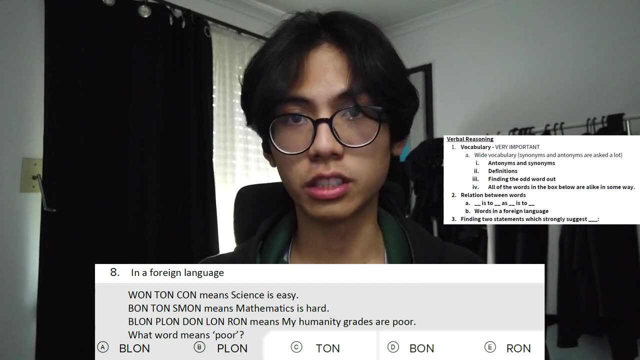 it's pretty much how they're gonna ask those types of questions. so it's important to know relationships, and then we have words in a foreign language which is going to be in a bit of a code, but this example question here again is going to showcase like what it's about, the last main. 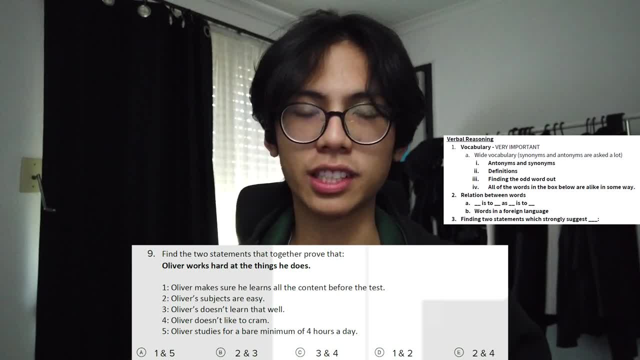 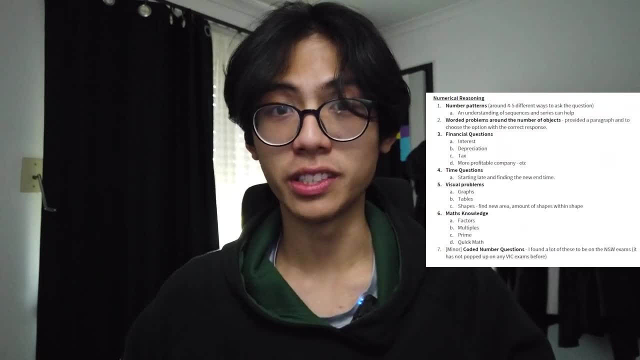 part that they always ask is find two statements which strongly suggest. so that means reading a sentence and then being given options to find the one that proves those statements. The last multiple choice component of the exam is numerical reasoning test. It's a bit of an IQ test that. 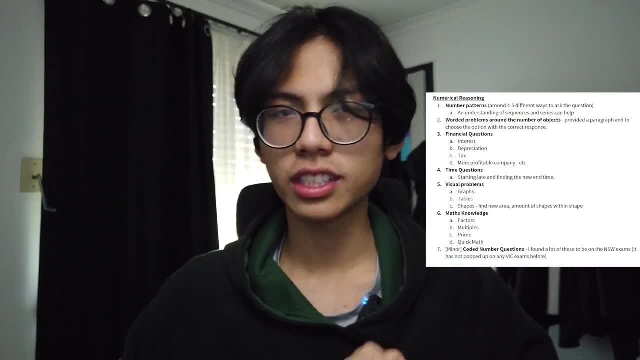 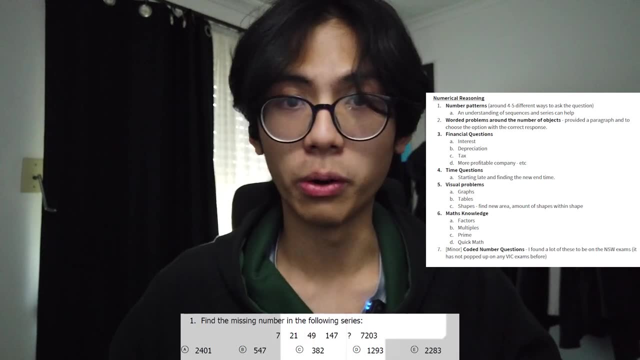 focuses heavily on number, pattern and relation. So I've broken this down into like seven key topics, although the seventh one is minor. So number one, number patterns. You're going to need to know how numbers relate and how they, I guess, either increase or decrease, depending on the situation. 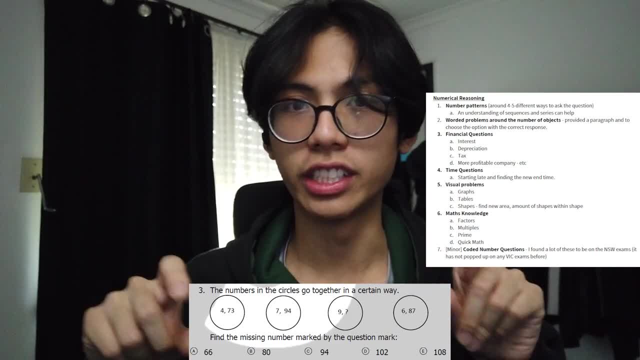 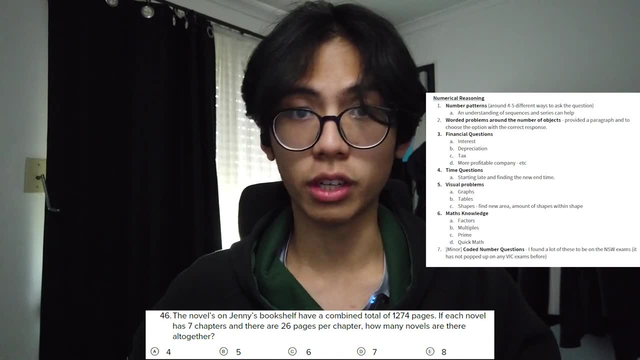 They're going to ask a question around find this number within this series or sequence. Then we have worded problems around the amount of objects. So you're provided a paragraph and are to choose the option with the best response that proves everything in the paragraph. Then we have 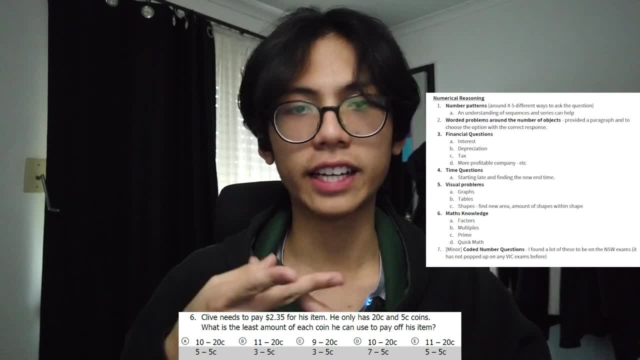 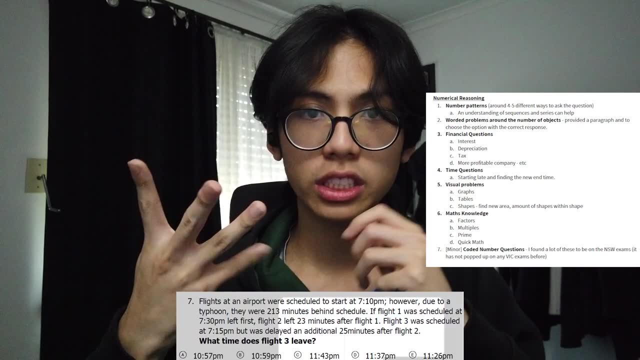 financial questions. So it deals with interest appreciation, tax, profit as well as like the cheapest thing or like the best value item. It really depends on the question. Then we have time questions, which are around starting late and finding the new time of things Like the example. 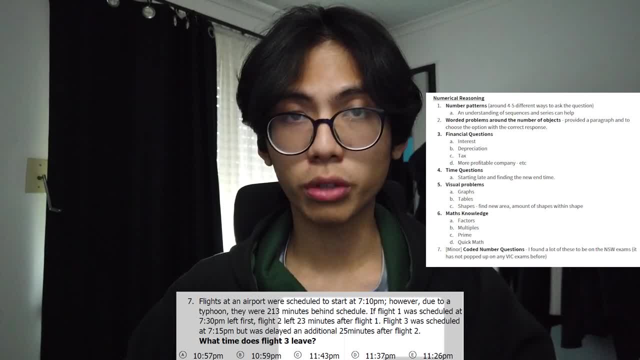 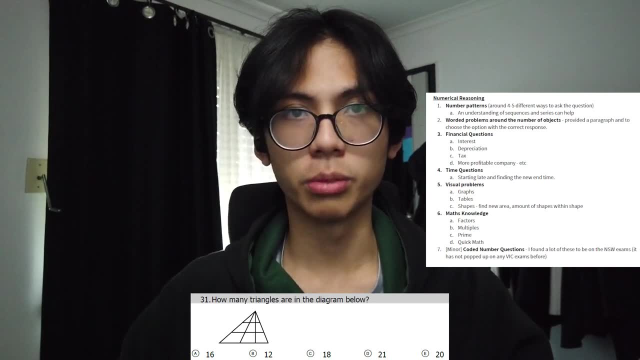 question here is probably going to show you that. Then we also have visual problems. So we're going to be given graphs and tables that you're might going to be asked questions about, or even shapes, which could be around finding a new area for the shape or finding the amount of shapes within one. 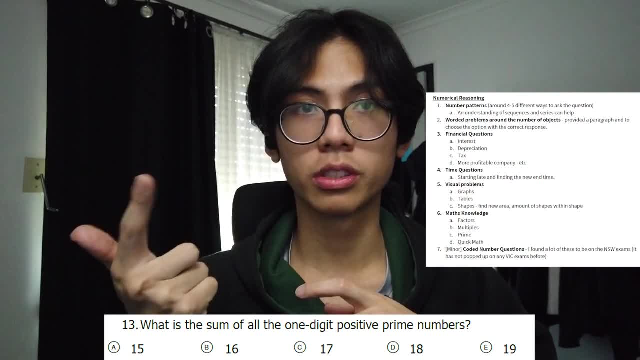 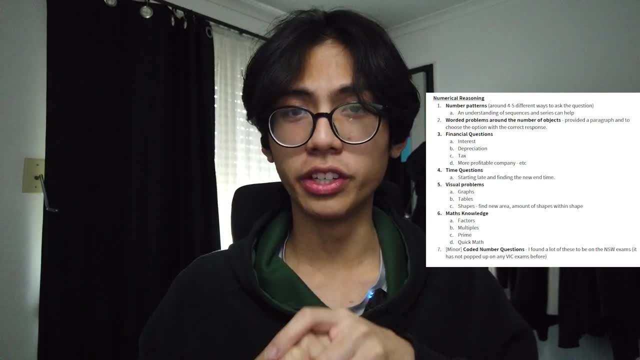 particular shape. Then maths knowledge: You need to know factors, multiples, primes and quick math. These four are going to be essential to like doing the exam in like a really fast manner. And then the last part is coded number questions, Although this hasn't really popped up too much on the 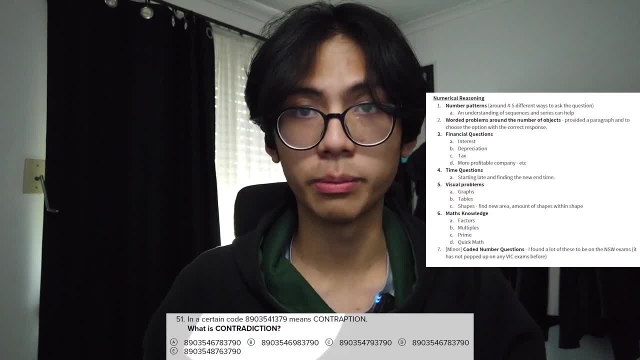 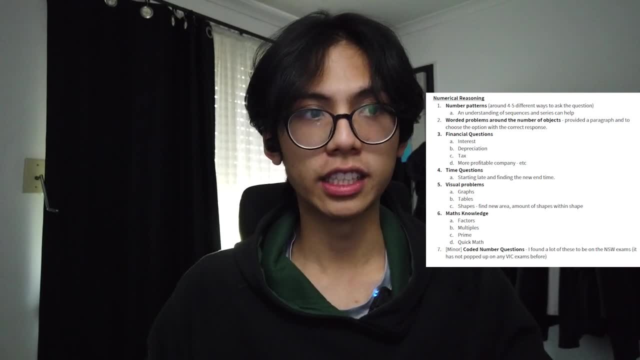 Victorian exams. it has popped up a lot in the New South Wales selective exam, So it is important to learn a bit, but don't worry about it too much if loose for time. And yeah, that pretty much concludes my checklist. I hope that the questions here that I share are like helpful to you as well. 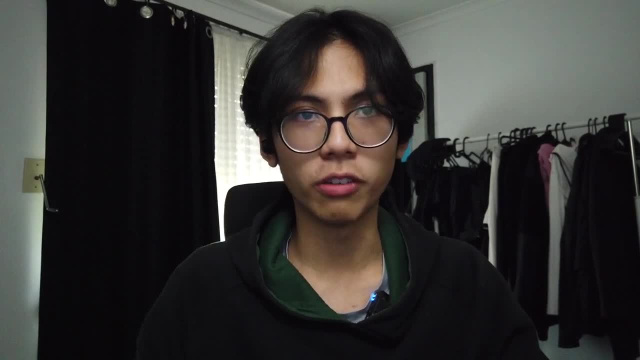 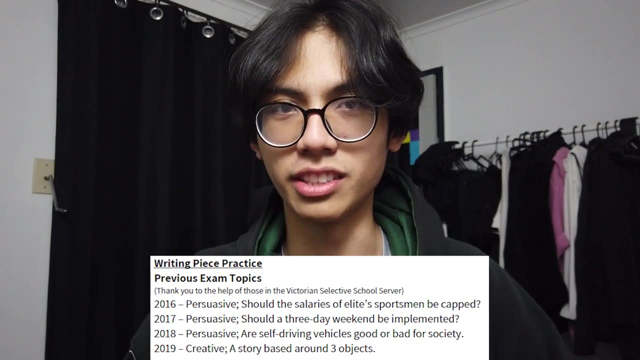 as just provide insights as to how my tests are, as well as what I offer Writing. There isn't much of a checklist to provide other than knowing the key skills like TEAL for essays and descriptive language for creative pieces. Instead, I've included the previous selective exam topic and 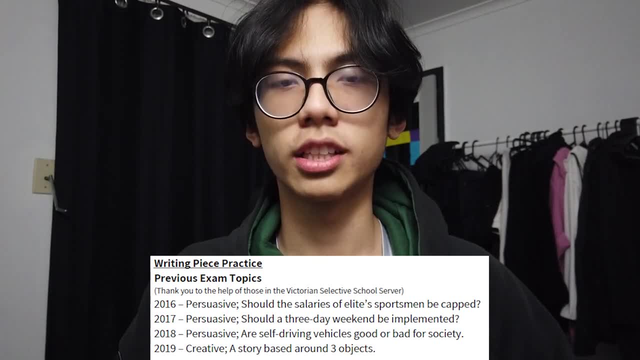 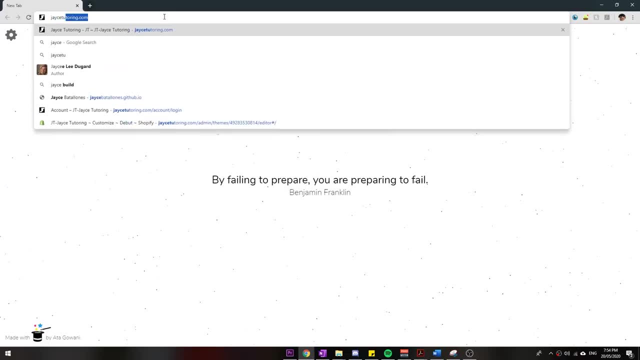 potential writing topics that you can practice. All the questions shown in the checklist came from personal tests that I've created and gone over with a couple of selective school students. Feel free to purchase the practice test PDF from the site on screen now. They're available for each of. 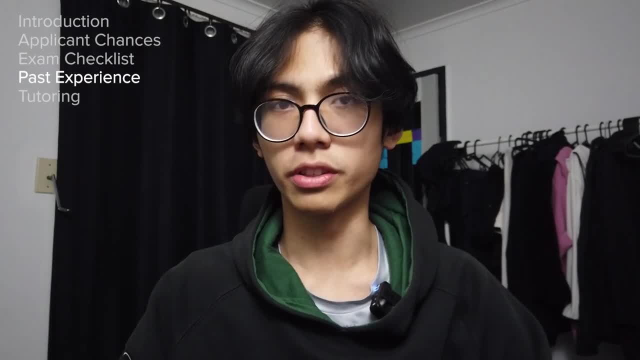 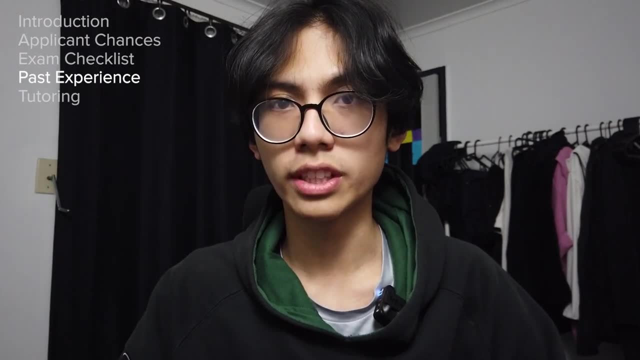 the exams and include all the multiple choice tests. Past experience: First of all, I did not actually sit the year eight to nine exam because I forgot to apply. I did, however, sit the Nossel and John Monash exams for year nine to ten, which include the same exam topic. I did Jack tutoring. 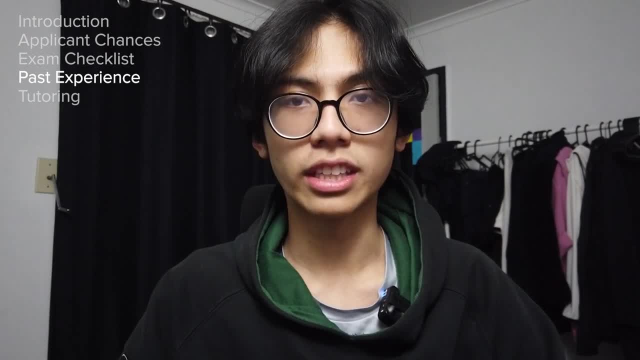 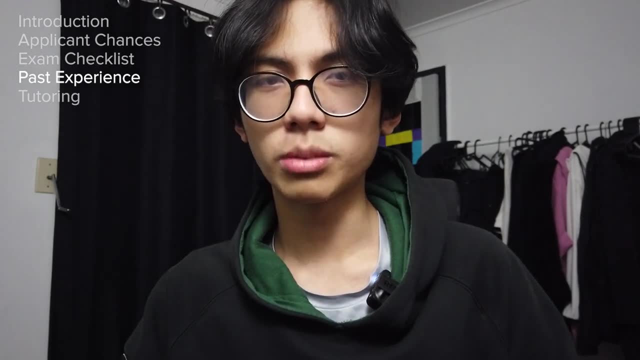 for year eight to nine because I plan to do the exam. I did Jack again for year nine to ten, specifically for John Monash, but didn't find it to be particularly useful when learning content. They didn't teach much and just spam students with practice tests, which were definitely helpful. 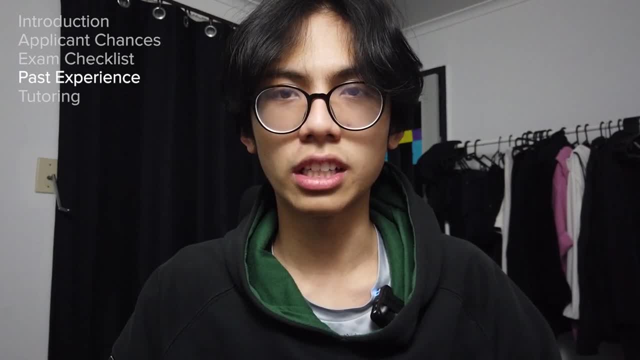 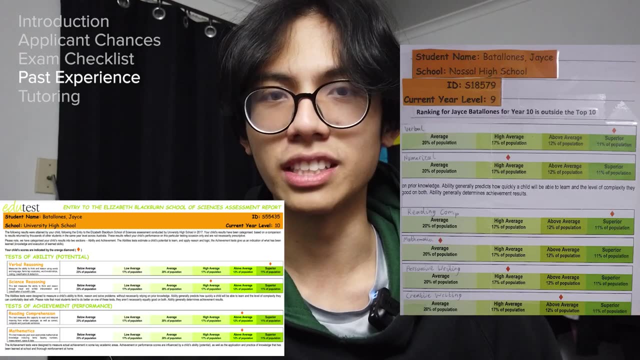 but not as helpful as they could have been, Since they gave back the marks, I usually was on the lower end of the spectrum. However, I managed to receive superiors on verbal reasoning and reading comprehension, despite my low scores, Having failed the first time and missing out by one superior or 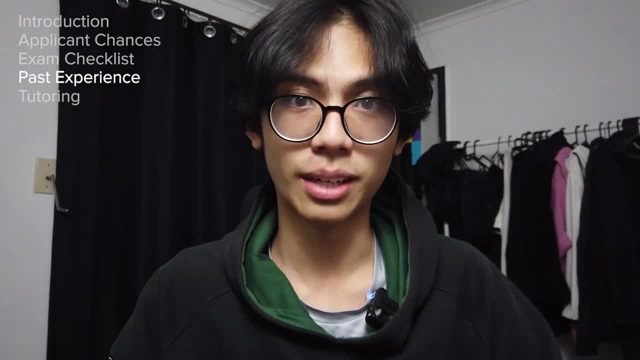 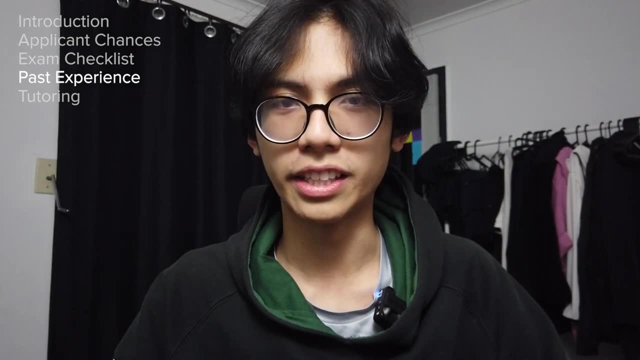 messing up the interviews, I once again decided to sit the Nossel and John Monash exams for year 10 to 11.. But I also sat the EVAS exam During this time. I instead opted for a one-on-one maths tutor and barely revised for English. 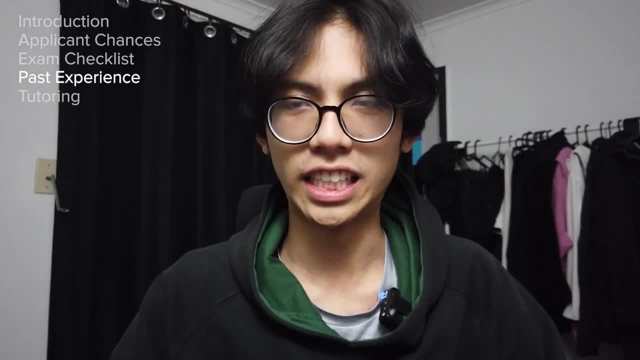 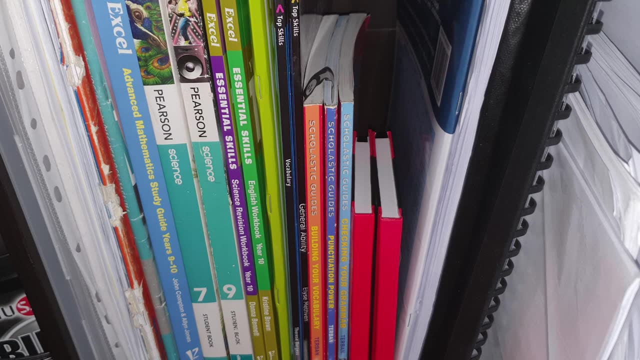 knowing that I could get superiors. Feel free to find out more about that in the. I failed the selective exams of Victoria in the card above. As for the resources that I studied, the ones in the image here are the ones I used in the past. Some are new which have been added to the. 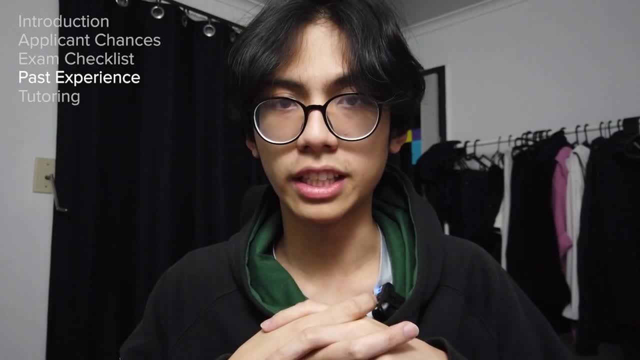 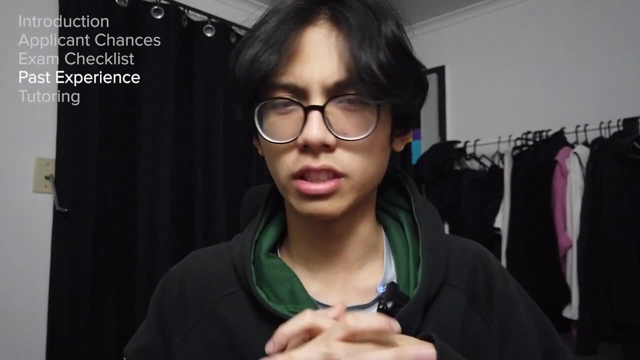 curriculum of my own tutoring program. I definitely recommend picking up a year nine to ten maths to improve your mathematics and numerical reasoning. I also recommend, like any of the Excel textbooks because they are created for the New South Wales selective exams, which pretty much cover the same content just in a different format. 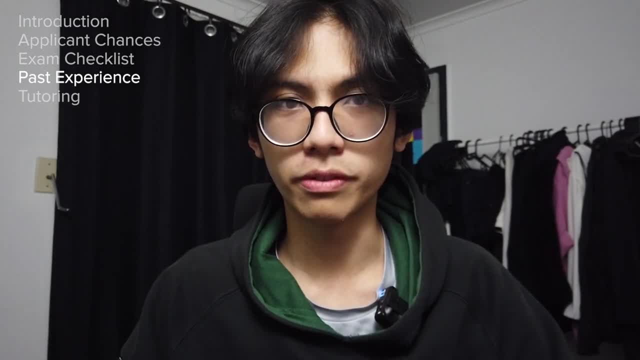 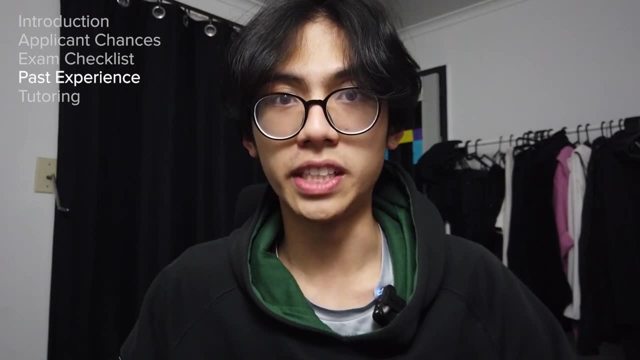 Before I continue, I want to say that you don't need to go to a tutoring program if you want to get into a selective school. All the information you need for the selective schools is provided in all the various guides and videos that either I make or others, So no program is needed. I do. 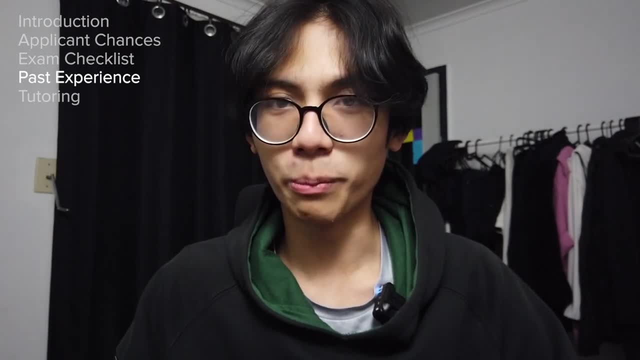 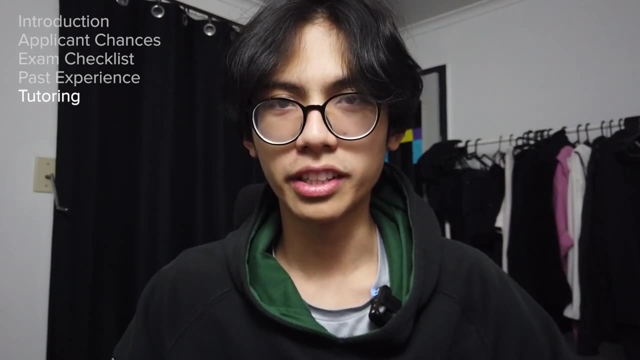 know a couple of friends who got into a selective by working their butts off or by applying from a same Thai school. It's really a matter of a bit of luck how badly you want it and how much work you're going to put in to make tutoring. If I was to recommend a tutoring program from the ones I 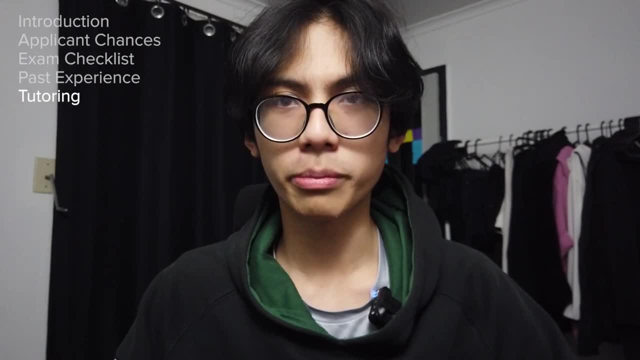 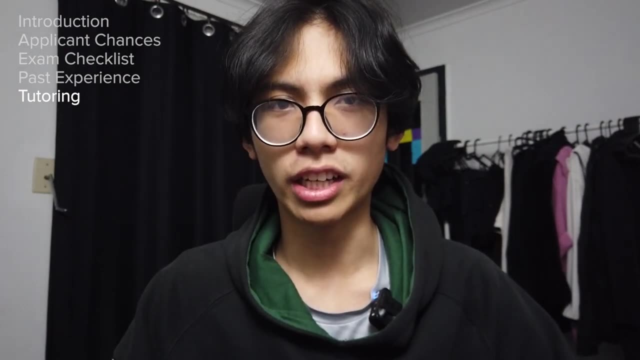 attended. I wouldn't recommend any. Instead, I recommend my own. If you want a program catered towards your own learning, my program is best for you. It is one that I have worked on for over the past year. I've been working and creating my own resources, pilot testing them on a small number. 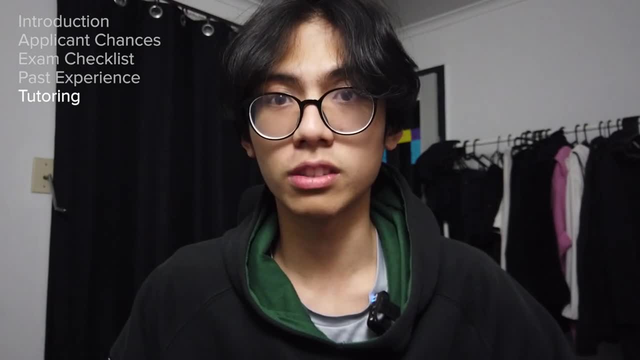 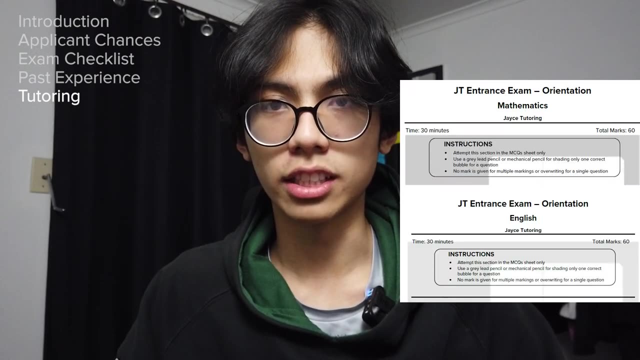 of students. Currently it has a 100% success rate for the science selective schools, but I have decided to branch out to all of them, since they pretty much cover the same content In the program. an entrance test is first sat to gauge the current skills of the student. It is 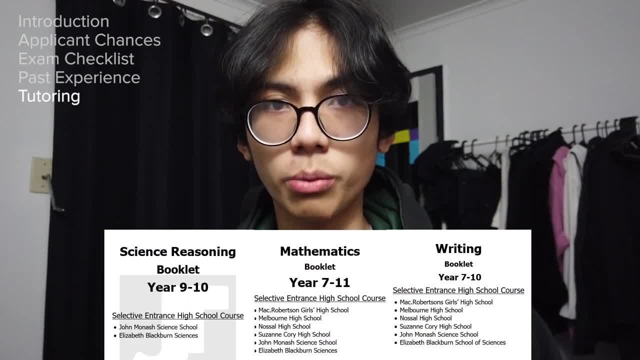 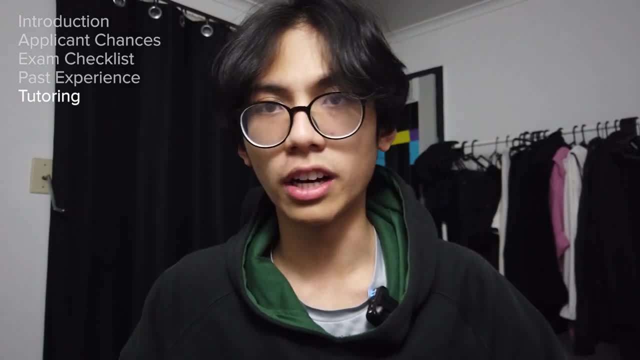 then followed by weekly lessons that teach the content for the exam, which is then followed by practice tests in the later week. My program has a heavy emphasis on accommodating the needs of the students, be it a slower learning rate, a faster one, sometimes even opting to just give them the 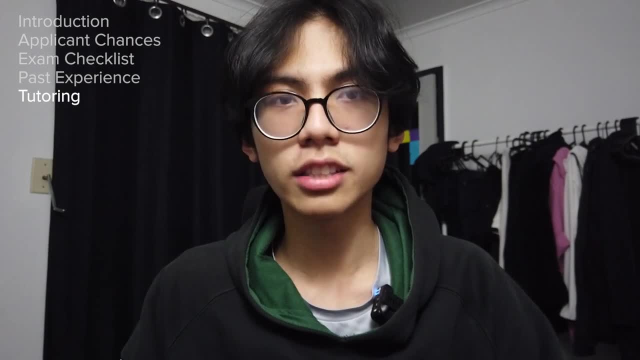 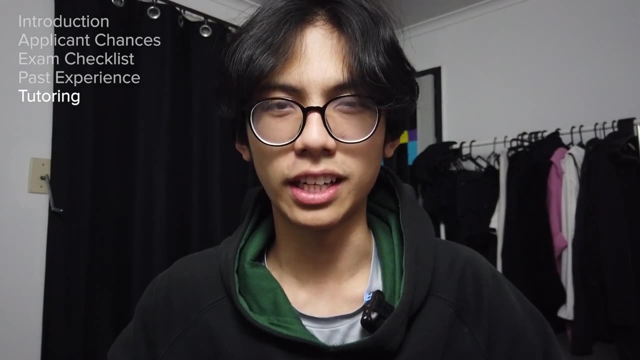 content booklets and letting them learn on their own. if they're like that, It is entirely dependent on the student as to how the lessons will unfold. Preferably, I'd like to have students query and answer the questions that they want to be answered, and I'd also like to have them answer the questions.